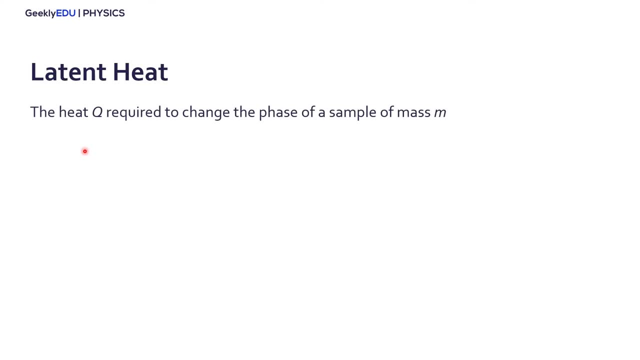 understand now the latent heat itself. so latent heat is actually the heat that's required to change the phase of a sample of mass. okay, as simple as this. you can calculate the latent heat by multiplying the mass of this fluid or gas or solid. multiplying by this L here. 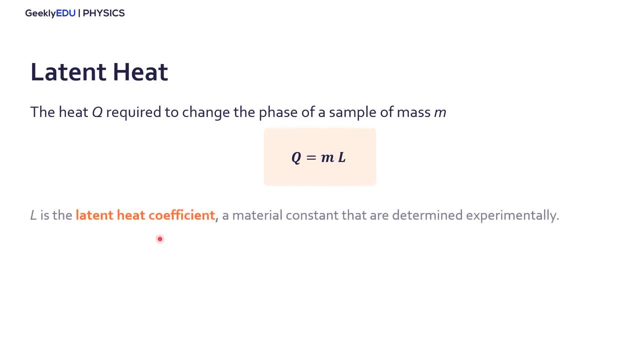 This L is a constant and it's the latent heat coefficient. That's a material constant that is determined experimentally. So depending on the thing you have, the material you have, you have different values for L, Also depending on the phase you are changing. 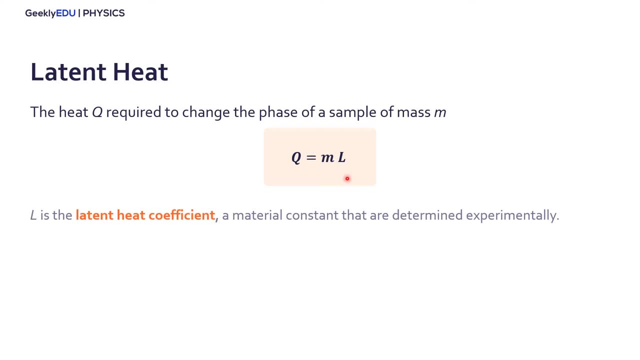 if you are going from solid to liquid or liquid to vapor, for example, for the same substance, the same material, this L here will also change. That's why we have the latent heat of fusion for melting and freezing, the latent heat of vaporization. 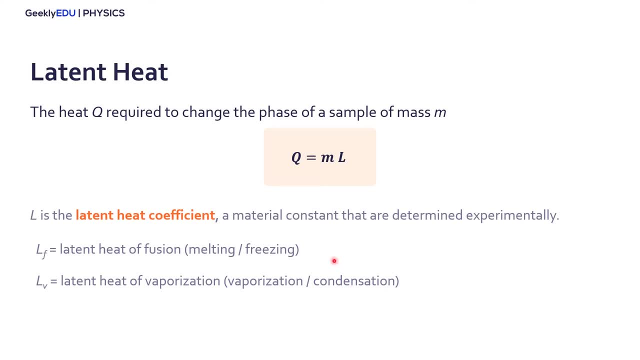 for vaporization or condensation, and also the latent heat of sublimation. Sublimation is that thing, that phase change that goes from solid directly to vapor or vice versa. So it depends on the material and the phase you are changing. 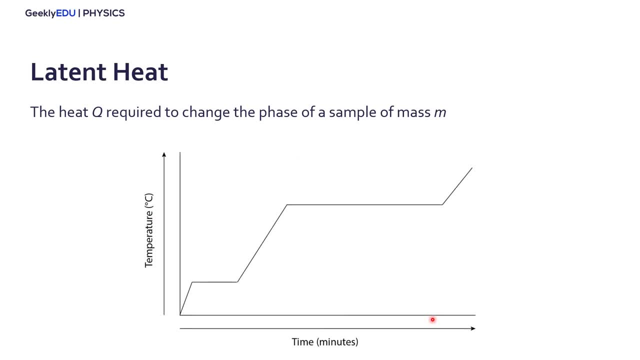 Simple, right. And another thing is that if we take a look here in this chart relating time with temperature, we can see that during the phase changes- again, it's very important- the temperature is constant. So every time you see a chart like this, 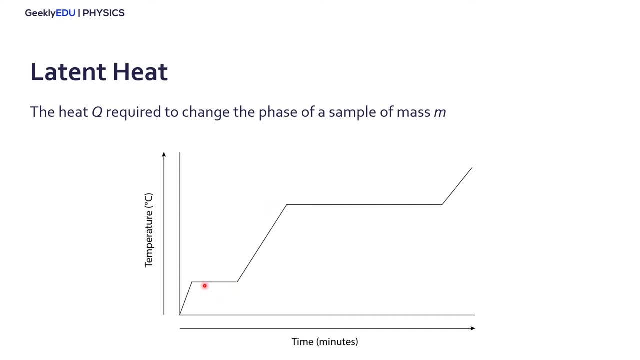 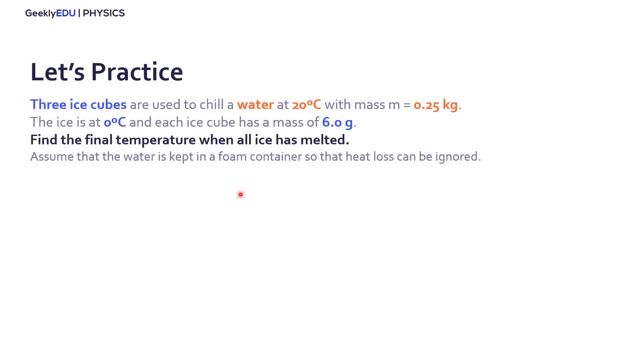 these flat parts. here are the phase changes, okay, Okay, so let's do this practical example. all right, We have three ice cubes that are used to chill water at 20 degrees Celsius, and this water has a mass of 5.5.. 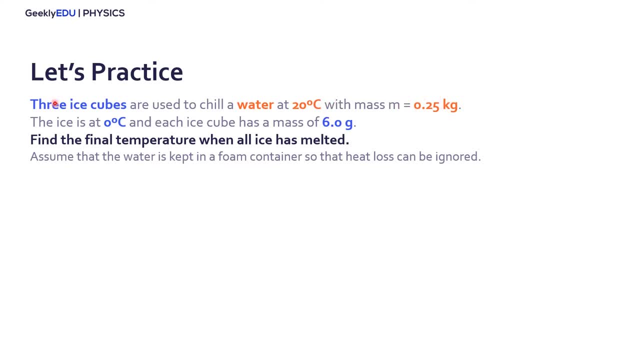 This water has a mass of 0.25 kilograms. The ice is at zero degrees Celsius and each ice cube- we have three in total, but each one has a mass of six grams. right, We want to find the final temperature when all ice has melted. 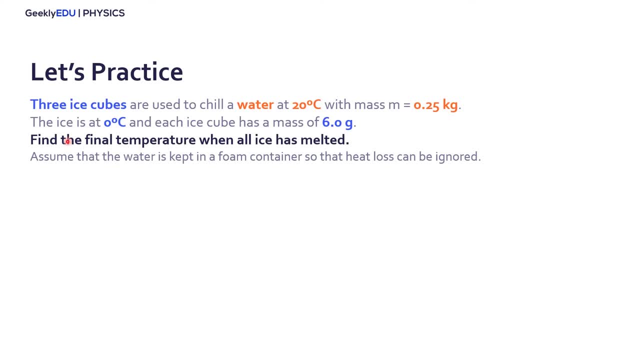 So we want to find the temperature at equilibrium. okay, So we also assume that the water is kept in a foam container so that the heat loss can be ignored. All right, there's no heat exchange from the water to the environment, just between the ice cubes and the water. 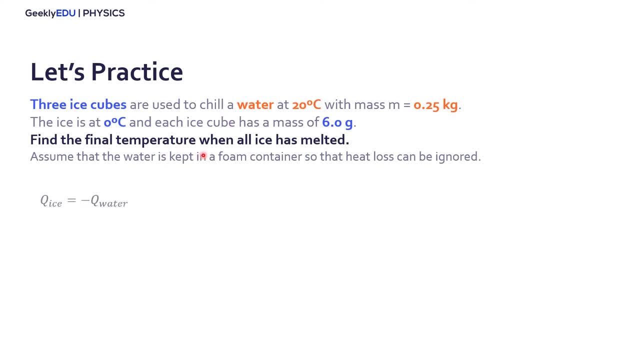 and we want to find this final temperature okay. So in the end, the heat exchanged from the ice needs to be the same that the heat exchanged from the water, So the water is cooling down. that's why you have this negative sign here. 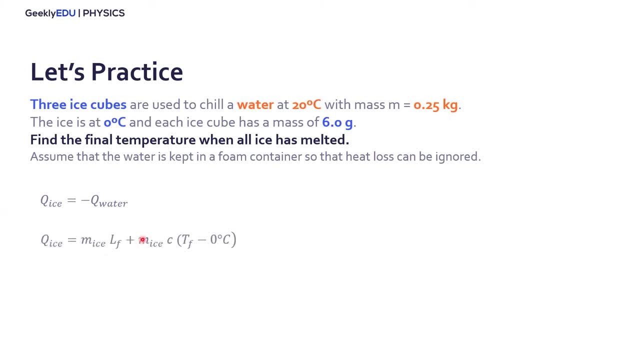 and the ice is warming up. So for the ice we have first a phase change from solid to liquid. okay, We are melting the ice, so we have the latent heat here, So latent heat of fusion. all right, We're melting. 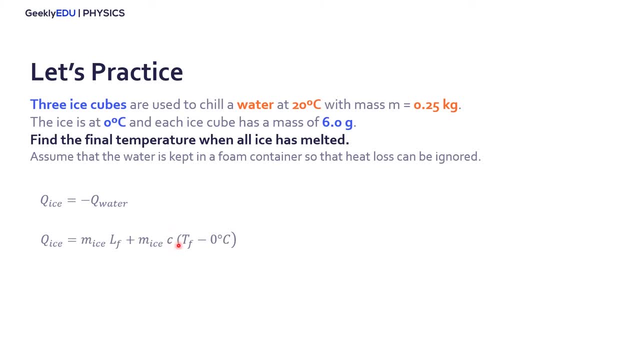 And also we have the m of ice times, C, specific heat times, the difference in temperature. If we're in doubt about this last part here, take a look in our video about specific heats, okay, So you understand it better. But basically you have the mass times, the specific heat of the ice. 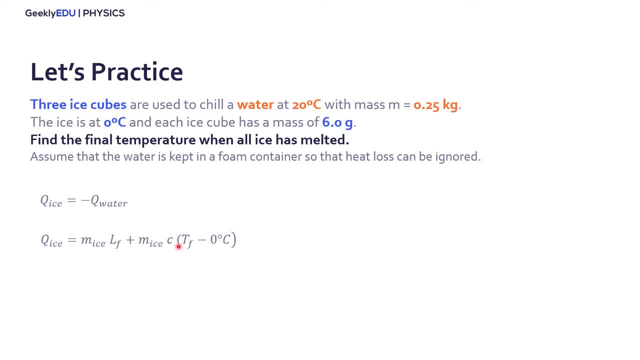 times the difference in temperature, the final temperature and initial temperature. We want to find the final temperature, all right, And that's exactly what's happening. okay, We have our ice, We have our heat. We have our ice here in blue. 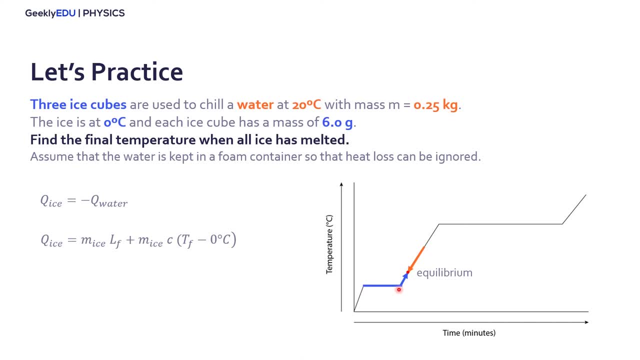 It starts at zero degrees and it changes the phase to liquid. That's why the temperature is constant, And then it increases a little bit. The water in orange here starts at 20 degrees and reduces its temperature until they find equilibrium. okay, Now for the water. we're just dealing with this change in temperature. 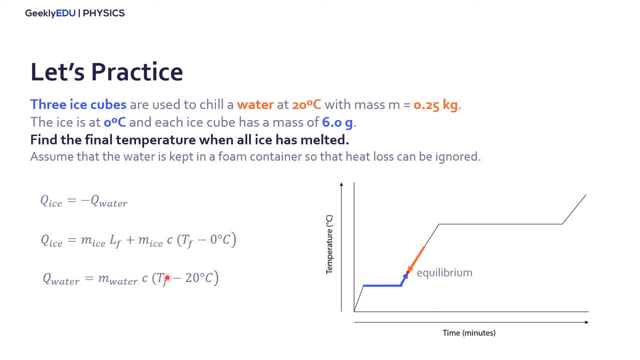 So we have m mass of the water times, specific heat times, the difference in temperature, final minus the initial. okay, Now you can just put this: say that these two equations here are equal, okay, And well, isolate the final temperature.